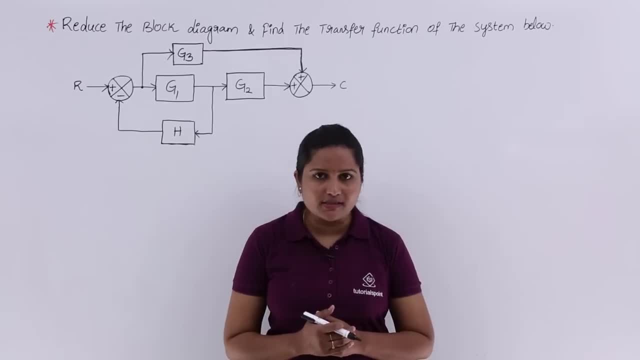 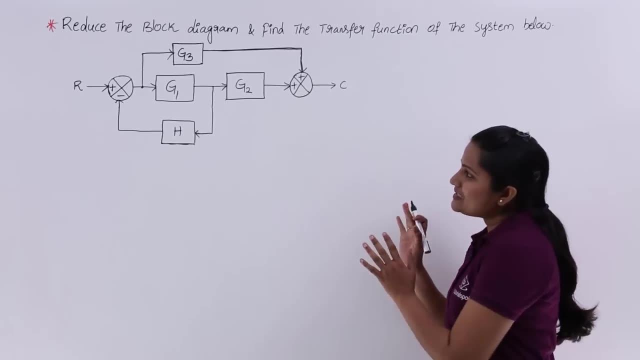 diagram and we need to find out the transfer function of the system. So you can see, reduce the block diagram and find the transfer function of the system below. So this is the system given, control system given. So we need to reduce this system and we need to find out the transfer. 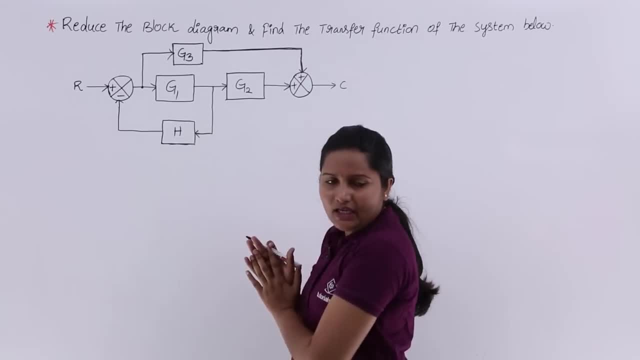 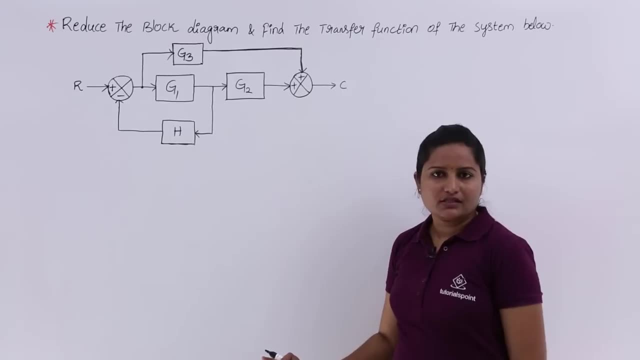 function, For example, at that, at this instant, if you want to find out the transfer function, how we will find out the transfer function? We do not know C of S and we do not know R of S. If you are having any single block in between C of S and R of S, you can consider that as transfer. 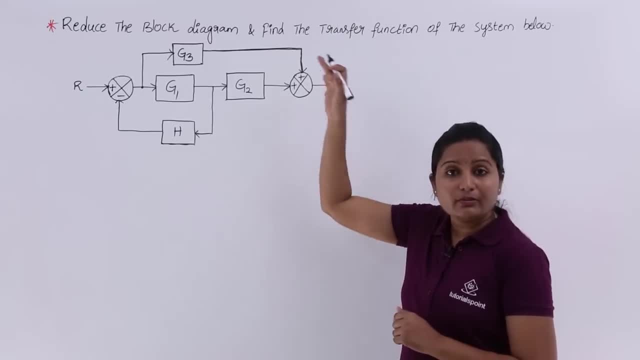 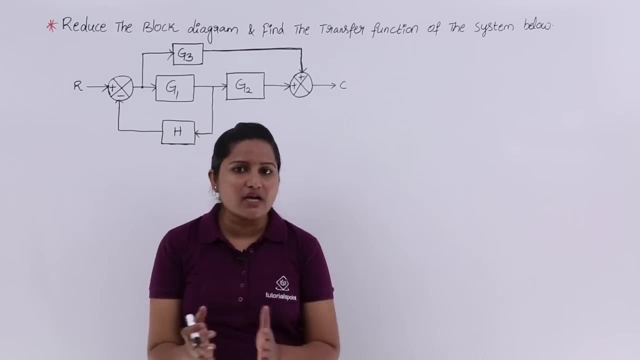 function of your system, but you are having multiple blocks. When you are having multiple blocks in between input and output, you cannot say that particular transfer function. So here we need to make all these blocks, all these different, different blocks, into a single block by using block. 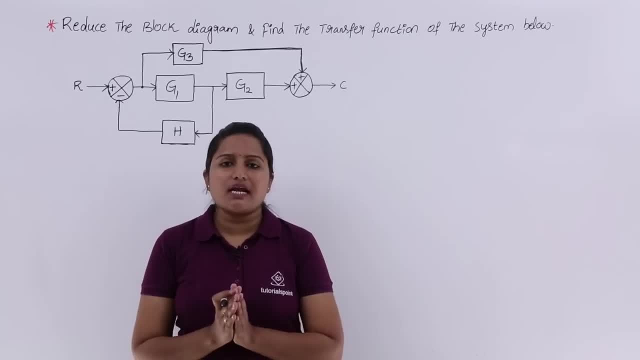 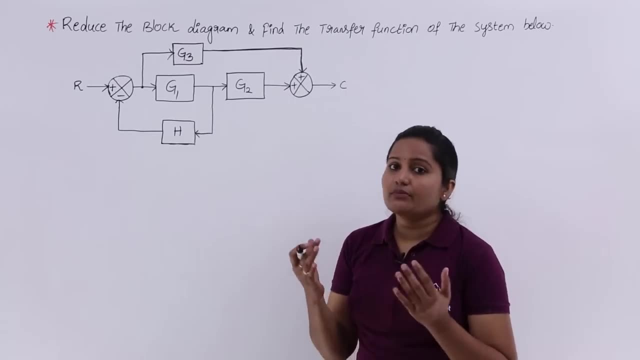 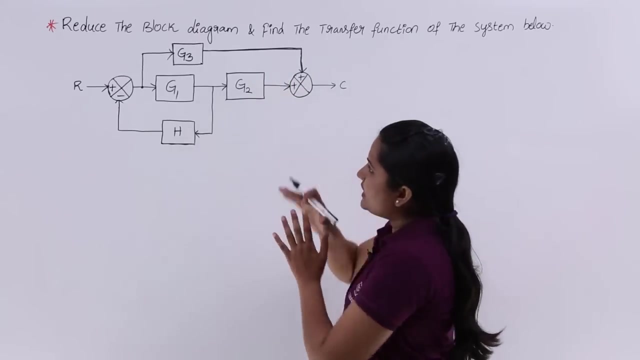 diagram reduction method. finally, that single block represents the transfer function of the system Coming to the reduction. in the last class itself we got some rules for block diagram reduction. So here you can see how we can deduct by observing itself. we are having some parallel blocks, we are having some feedback path and we are having some series which which? 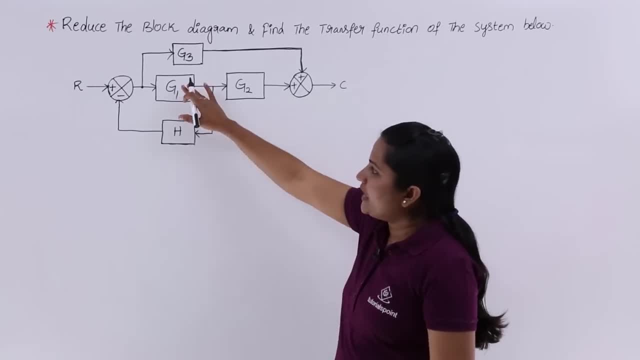 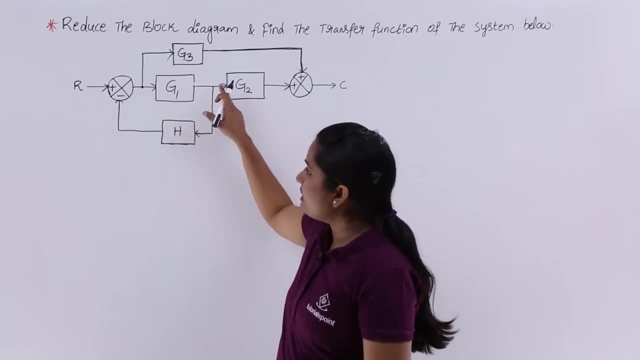 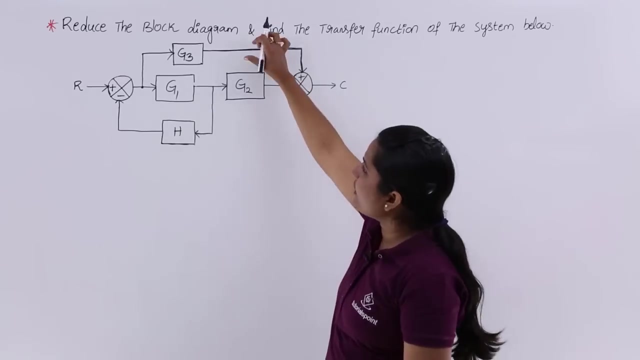 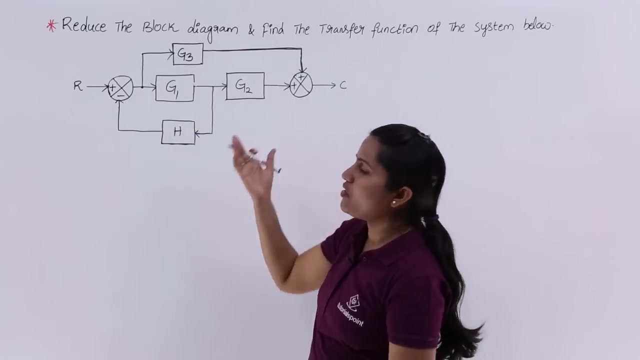 part we need to reduce first. For example, if you want to reduce the series path here, this series element is in feedback width, This feedback loop, So we cannot. If you want to reduce this parallel element, So here also in this parallel path, if this feedback is not there, then definitely you can write. 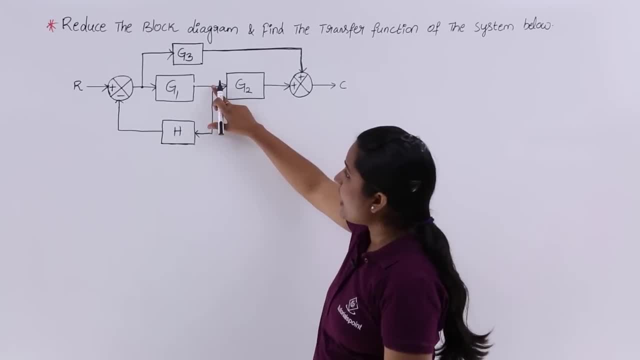 G 1 plus G 2 plus G 3, but here you are having a disturbance due to this feedback path. So, because of this feedback path, you do not know the effect of this feedback on this gains. So that is why you cannot. 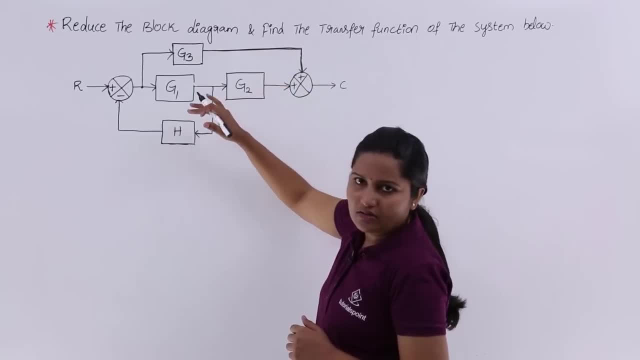 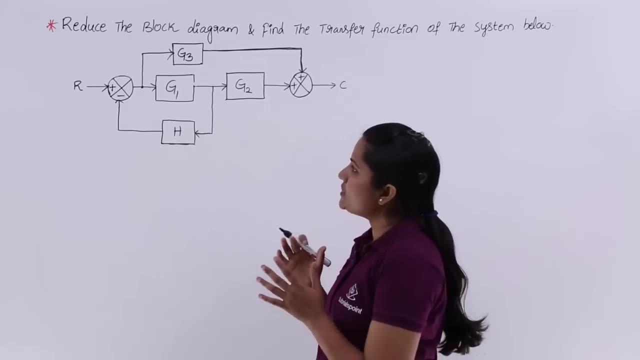 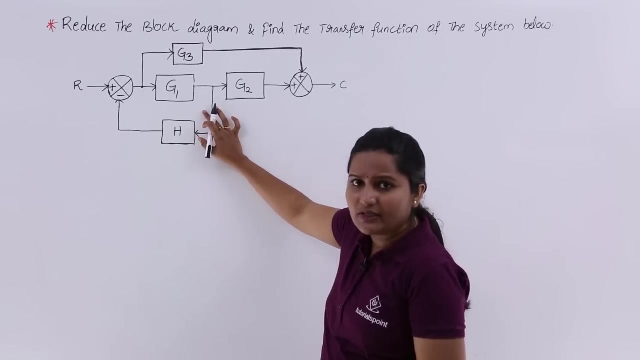 do this parallel block reduction also. you cannot do this first, you cannot do this parallel block reduction first. So which we need to do, for example, if you want to do this feedback, so that is also not possible first. why? because so in this feedback path, this branch point is included. 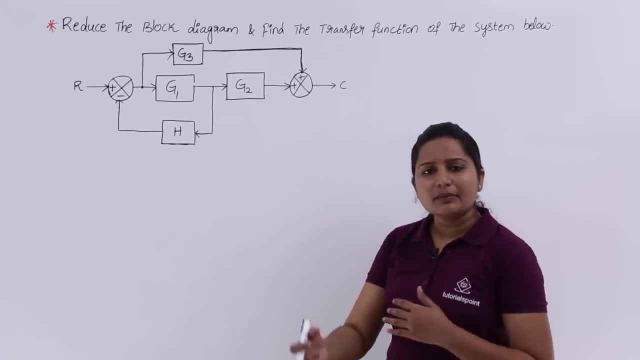 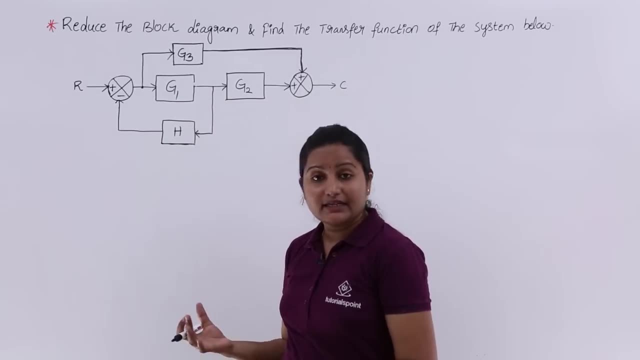 So we are having disturbance from other points. for example, here is: you are having feedback loop. if you can reduce that feedback loop, then that will be better, but you are having branch point here. Whenever you are having branch point here, if you feel that. 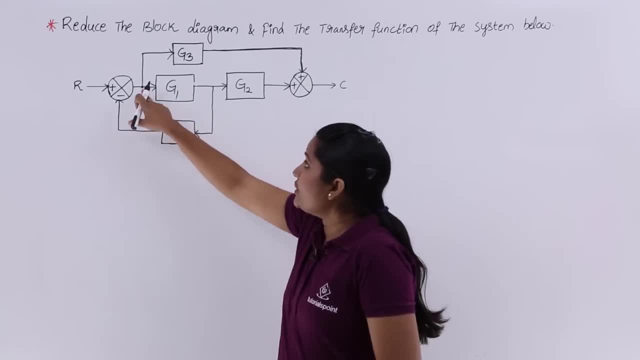 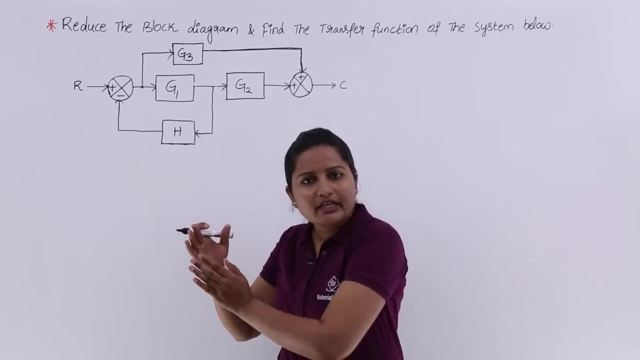 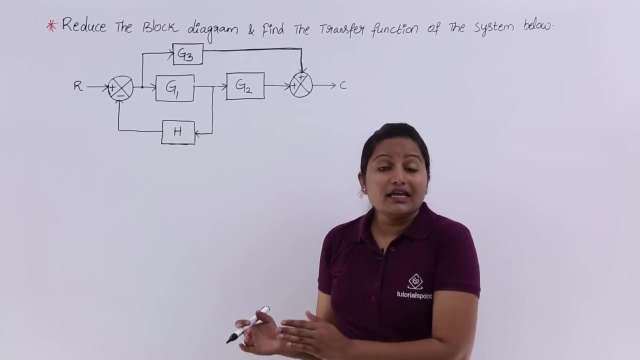 branch point is a circle to you, then you can move that branch point to here. So we are having a rule to move any branch point to ahead of the block. When you are moving any branch point ahead of the block, then you need to multiply reverse gain of actual path. you need to add a block. 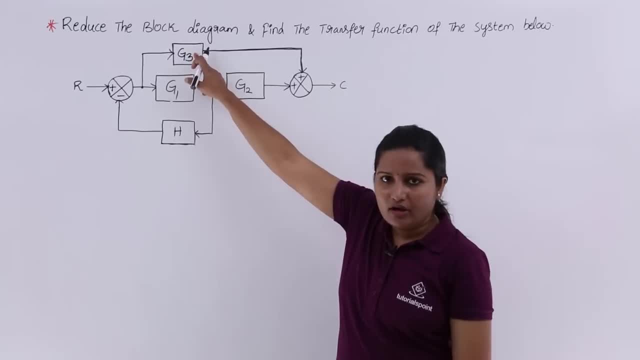 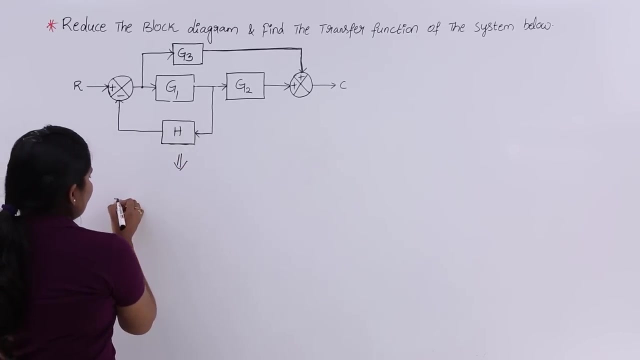 when block is not there already. we are having block here. no need to add extra block. for this block gain, you need to multiply reverse gain of your actual path. So you can see I am modifying my block diagram like this. So here I am having a summing point. 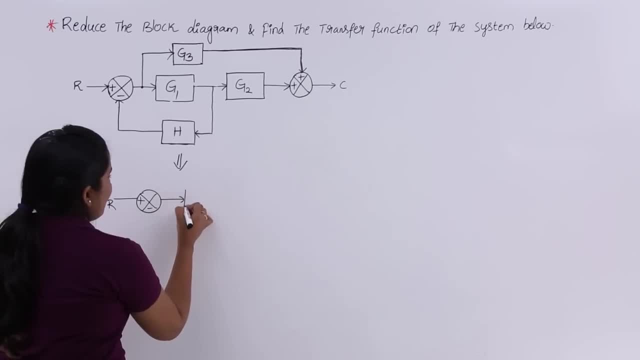 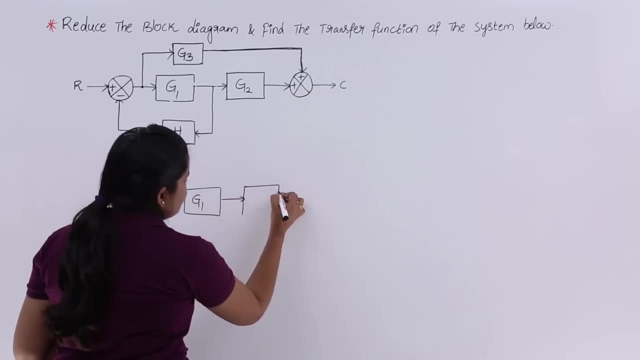 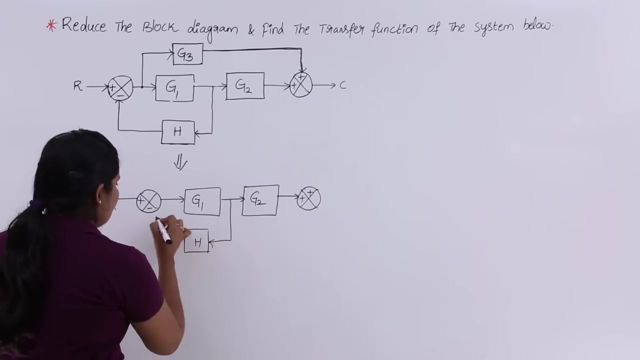 this R, and here I am having G 1, here I am having G 1, and here I am having G 2, my G 2, like this, and here I am having another summing point like this, and here, from here to here, I am having a feedback path, feedback path. So you can see, what I need to do is So. 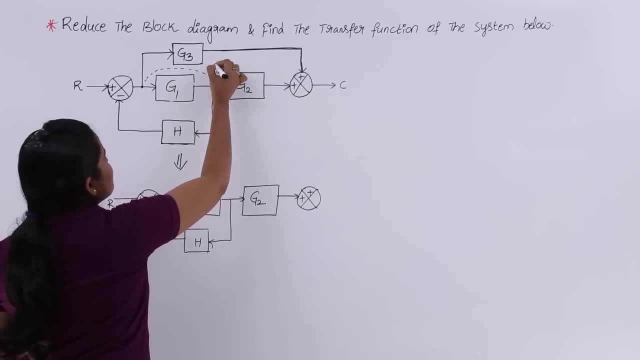 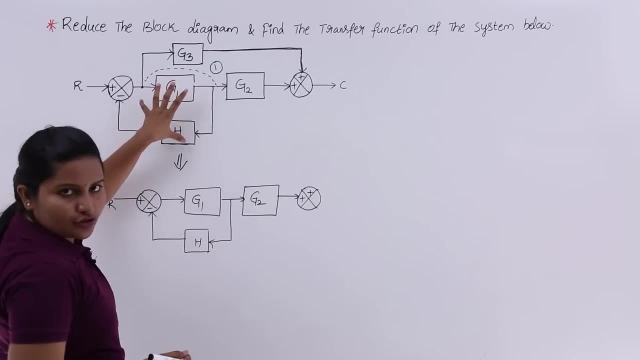 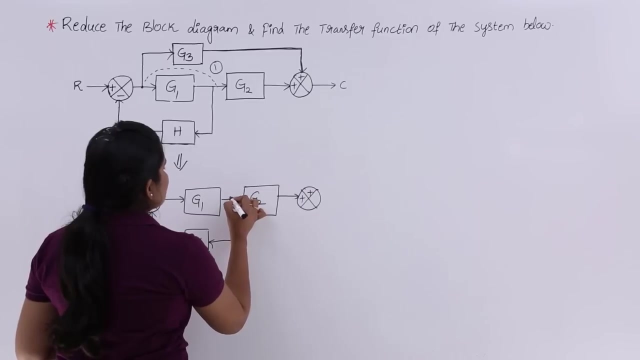 I am moving this branch point to here. this is the first step I am doing. I am just moving this branch point to here to simplify this feedback path. So here I am moving this branch point to here. So the gain will be modified as G 3 by G 1.. If G 3 is not there, if you are having empty, 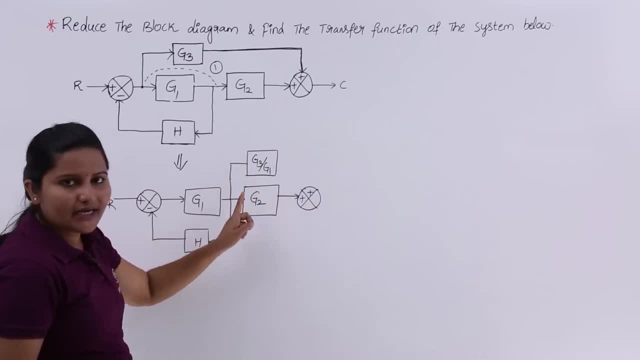 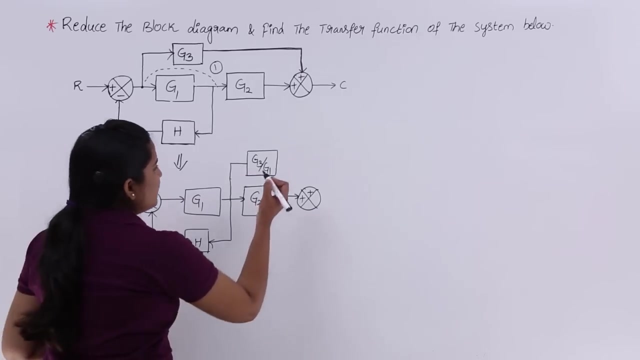 line, then you need to add a block and you need to write 1 by G, 1.. If you are already having block, then for that block gain you need to multiply the inverse gain of this ahead block. So here I moved this branch point to here, and here I am moving this branch point to. 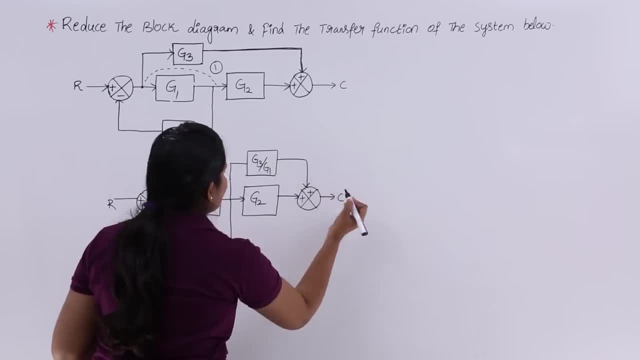 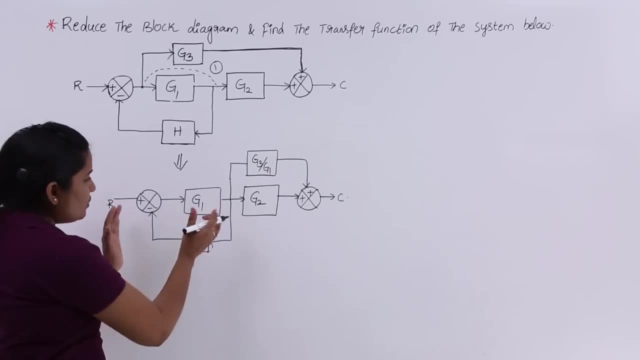 here. So here I am moving this branch point to here, and here I am moving this branch point to here. So I have got this point like this. So you can see, now to reduce this feedback path, I am not having any problem. So in the next step I am reducing this feedback path. 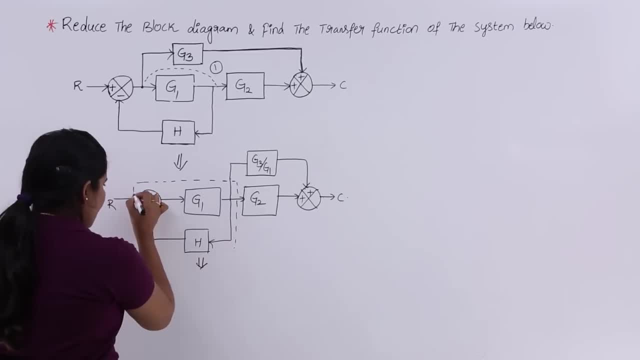 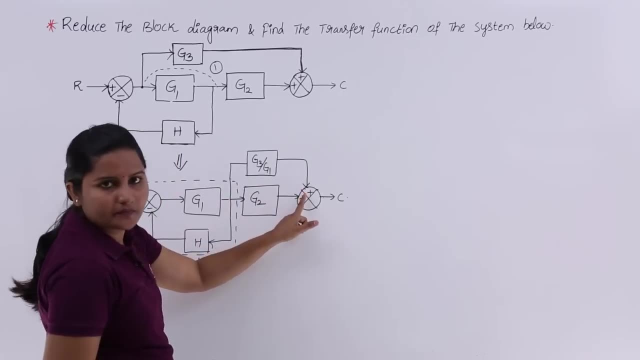 So, for this feedback path, I am writing like this: and here, if you observe, these two are in parallel. So, and these two are in parallel, So in the next step, I am writing G 2 by G 1.. So G 2 by G 1 is equal to G 2. this is equal to where I have in this line and G 2. 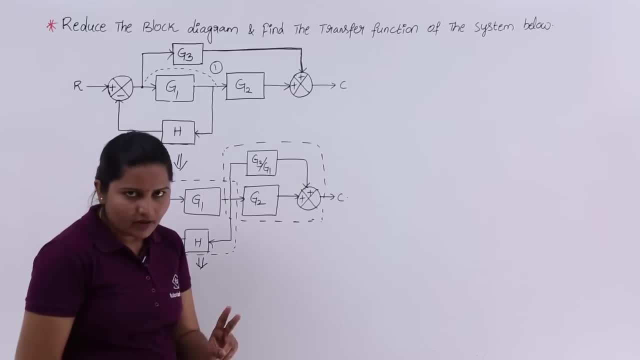 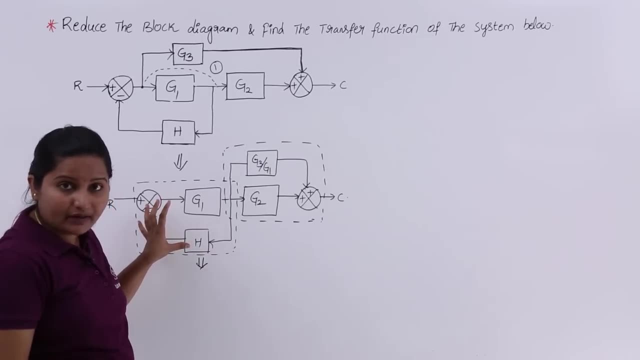 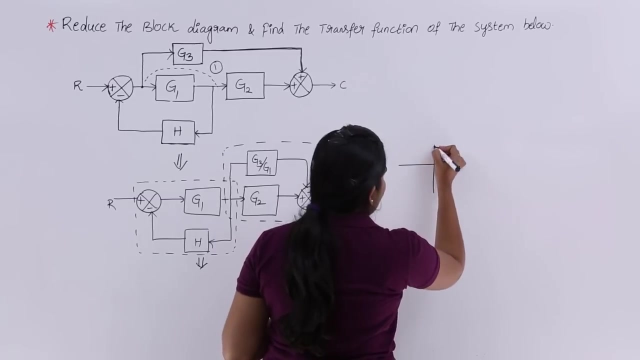 So in the next step, I want to do two things. one is I want to simplify my feedback path. I want to reduce my feedback path as well as I want to reduce this parallel gains, So my resultant diagram will be like this. So here, I reduced this feedback path, so you need to see which feedback 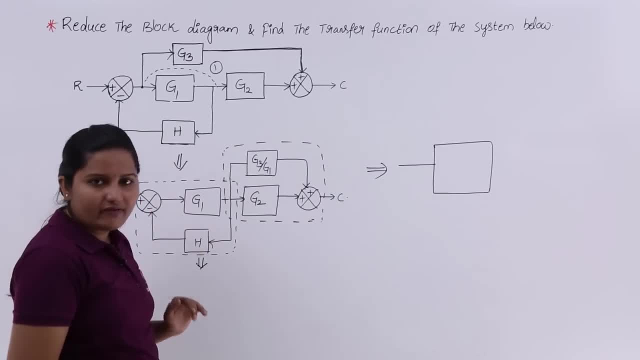 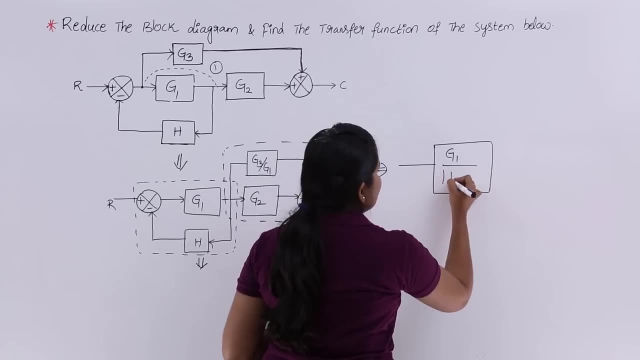 that is, that is a negative feedback. So g by 1 plus g h formula we need to take, as we are having g 1.. So g 1 by 1 plus g 1 into h. this will be the feedback path gain after reducing. 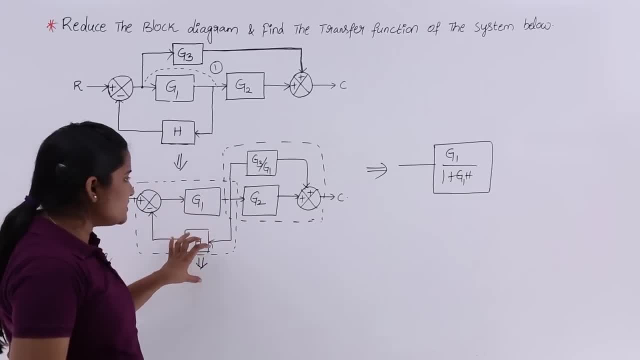 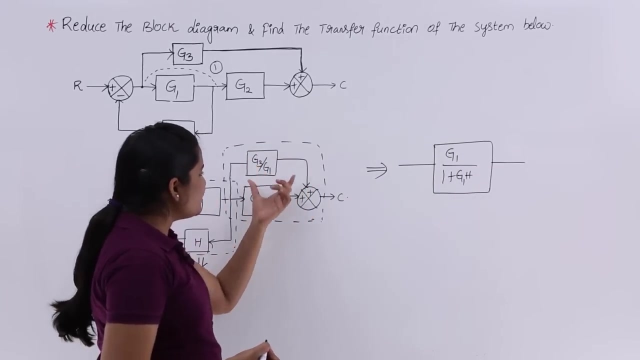 So no need to take the summing point and these two open loop gain and feedback path gain. So in place of these three, we can replace this block. So I reduce the feedback And now my term is to reduce these two elements. These two elements are in parallel. How we 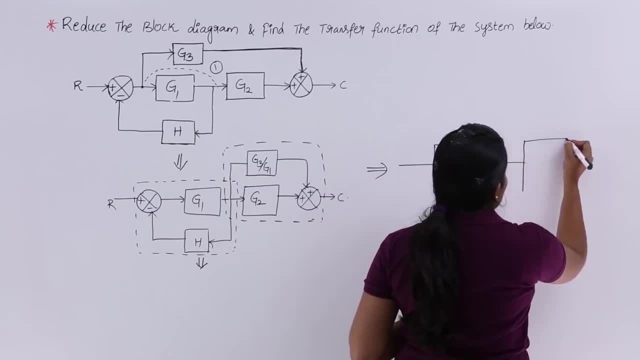 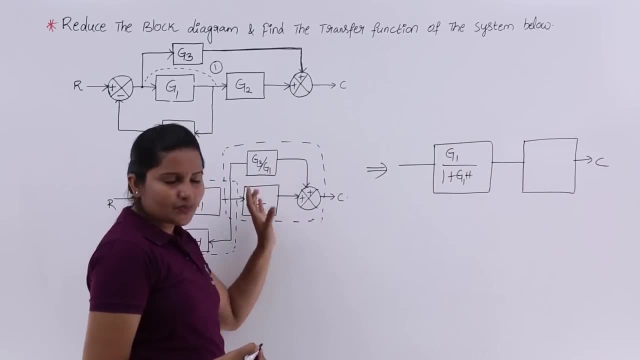 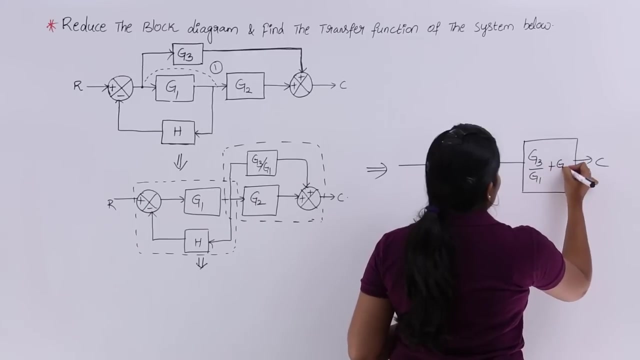 can reduce the parallel elements. by just adding the gains, we can reduce the parallel elements. So what are the gains? means: g 3 by g 1 is one gain plus g 2.. So this is equivalent to g 3 by g 1 plus g 2.. So now my block diagram is like this. So now, 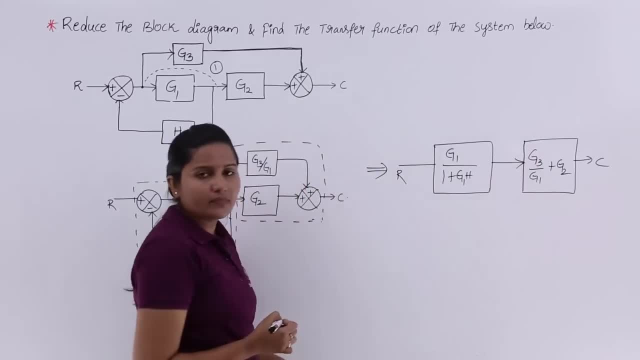 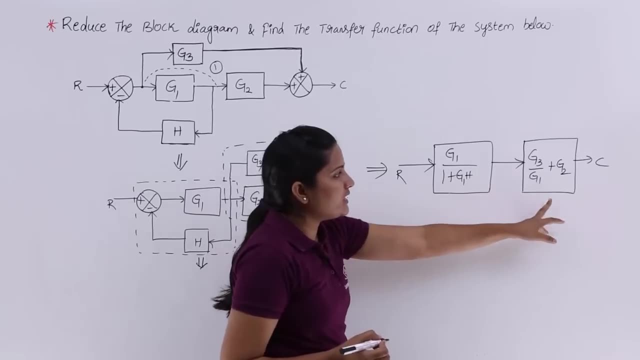 you can see that the block diagram is reduced to like this. So if the two block that are given is not enough, two block are given. now also I am not having single block, Now also I am having two blocks. So here you can see, these two blocks are in series. So if these 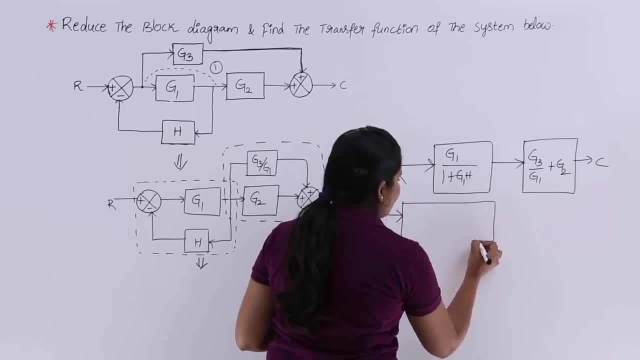 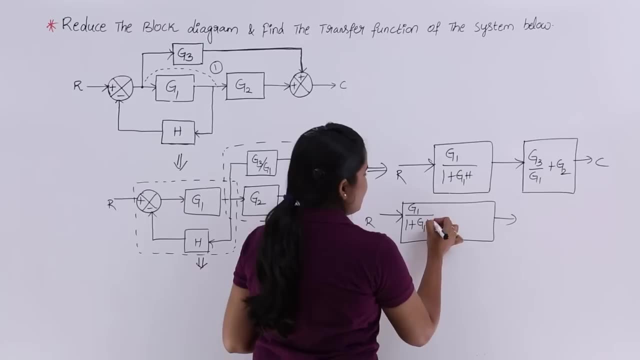 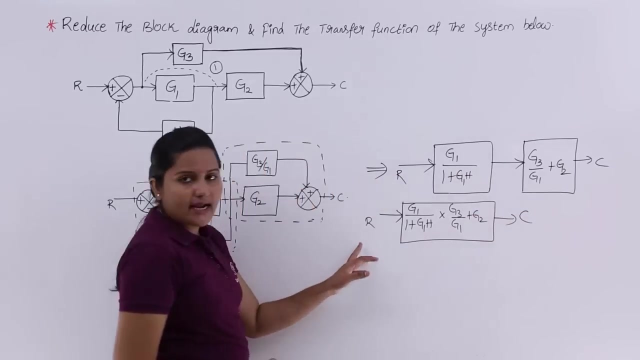 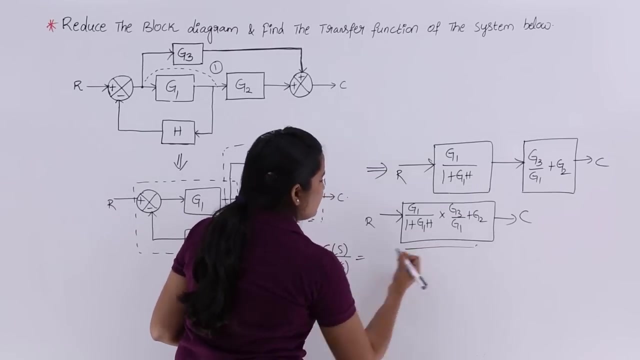 two blocks are in series. you can multiply the gains to make this as single block. So plus G 2.. So now the transfer function C of S by R of S is nothing but this gain. So G 1 by 1 plus G 1 into H, So multiplied with. so I am cross multiplying these two G, 3 G. 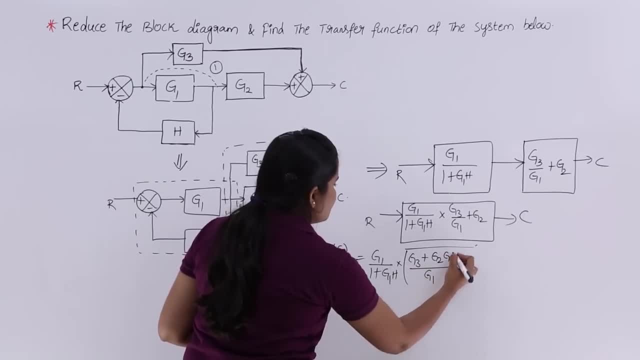 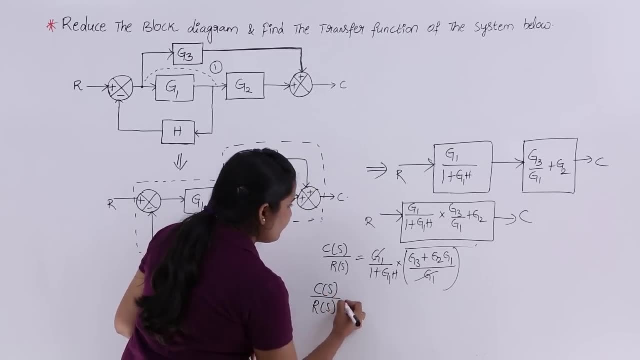 2 G 1 divided by G 1.. So I am cancelling these two. I am going to get my transfer function C of S by R of S is equal into G 1, G 2 plus G 3 divided by 1 plus G 1. H. This is the transfer. 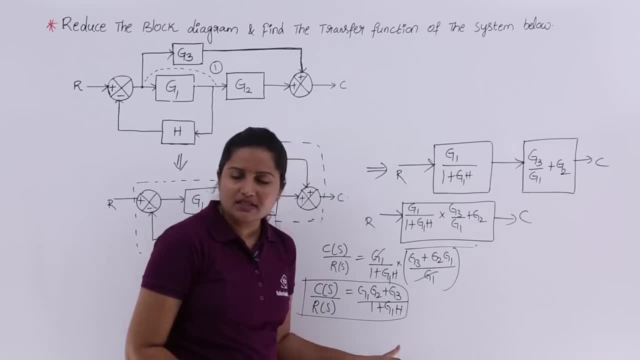 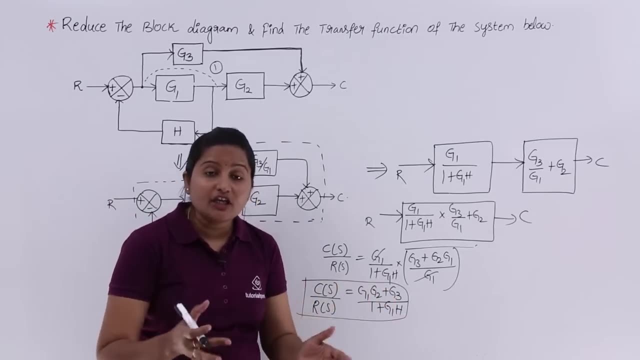 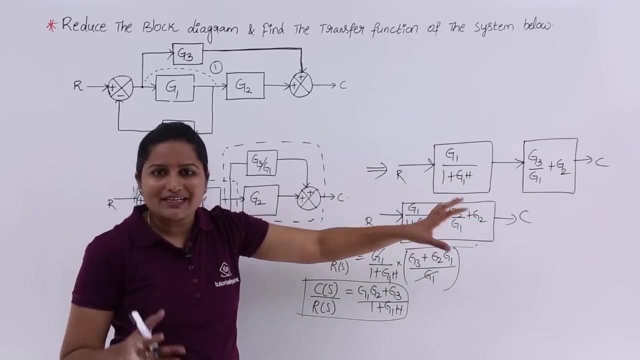 function of the given block diagram. This is the transfer function C of S by R of S. What we need to do when they are asking transfer function means we need to reduce the bulky block diagram into single block. So in between input and output that block gain will represents the 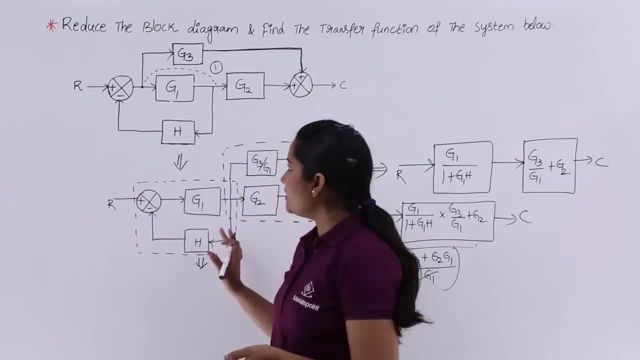 total gain. So that is the transfer function. So in between input and output that block gain will represents the total gain or transfer function of the system. So here I felt this branching point is some abstracted to me, So that is why I moved to here after moving. 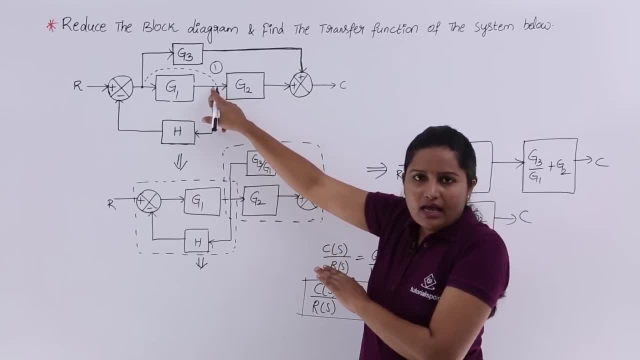 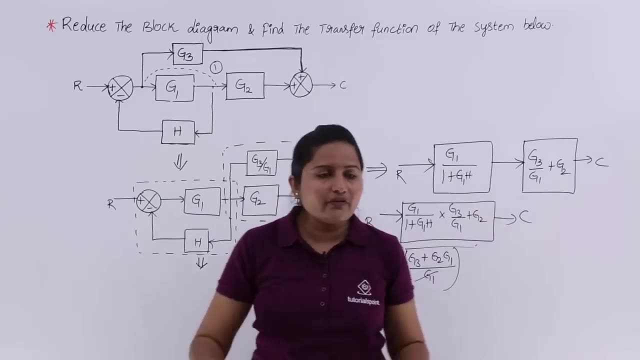 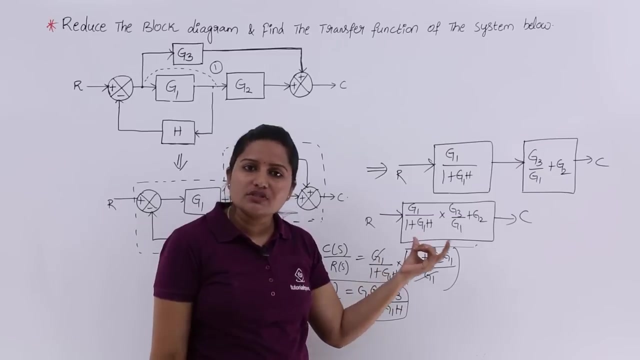 that branch point to. ahead of that, G 1, I got an idea to reduce the feedback loop and to reduce the parallel elements. After reducing feedback path and parallel elements I got two gains in series. So by multiplying that two series gains I got a single gain. So 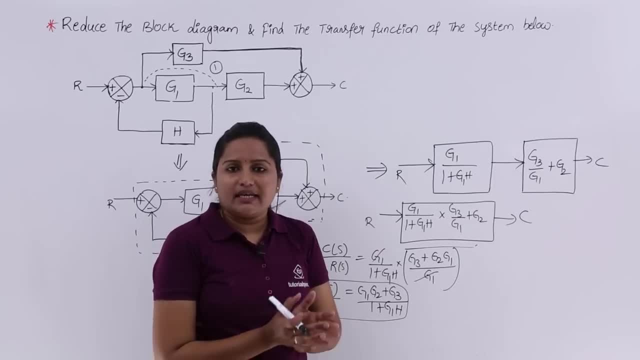 that single gain will be the total gain of the system or transfer function of the system.